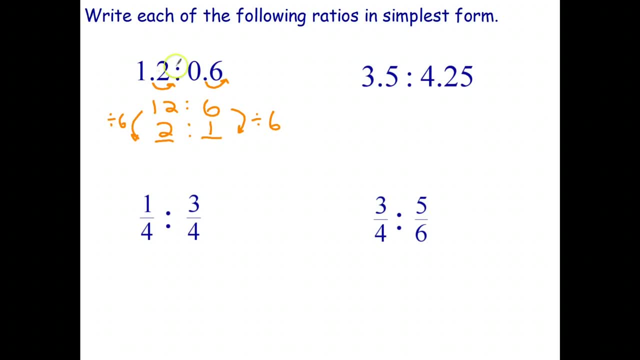 And that's certain. We don't want to discourage students that have good number sense and say, oh, you can't use that, So therefore you have to show all the working. So I would think in my case I'd be quite happy if a student just wrote that answer. 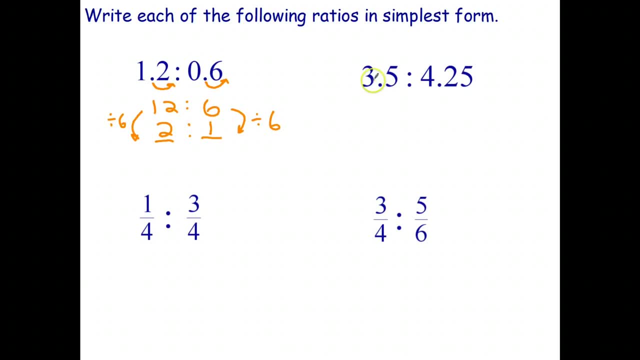 Okay, let's have a look at this one. Okay, here we have just one number after the decimal point, Here we have two numbers. So here we're going to have to multiply by 100 in order to get rid of that decimal point. 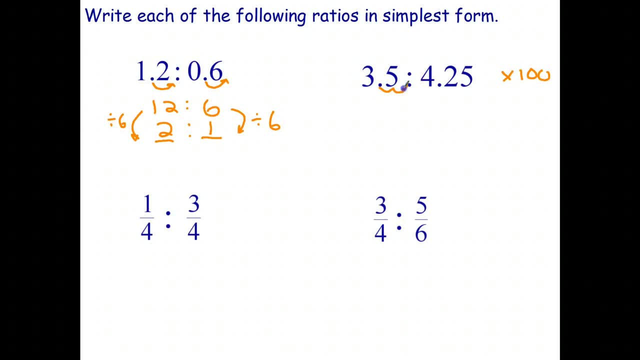 So move the decimal point two places to the right And that means we're going to have 350 there. Move that one two places to the right and we get 425.. Well, I know that 25 goes into both of these. Let me try this in my head. 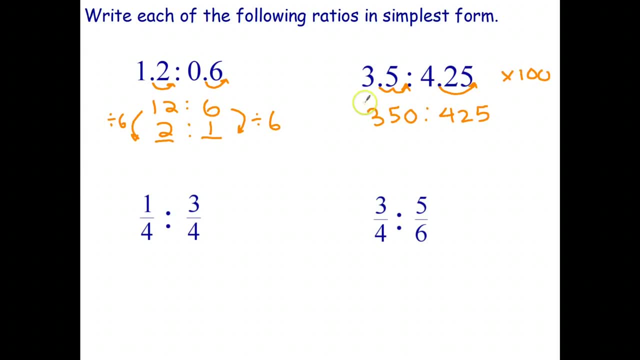 So 425 is 100. So 300 is going to be 12 and another 2. That gives me 14.. So what I'm doing here Is dividing by 25. So you can use a calculator if you wish to. 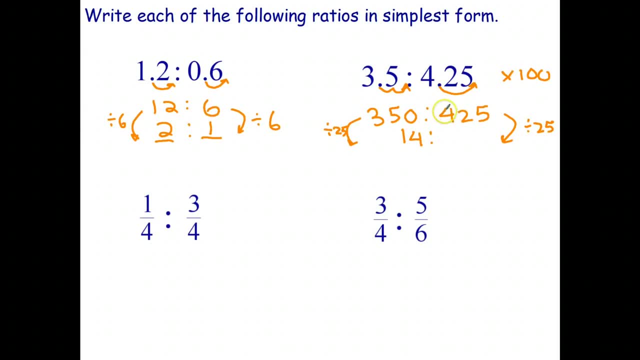 And 425 is 100. So 400 is 1625, plus one more is 17.. And 17 is a prime number. So that's not going to simplify And 14 is not a factor of it. So therefore, 14 is to 17 is the simplified ratio. 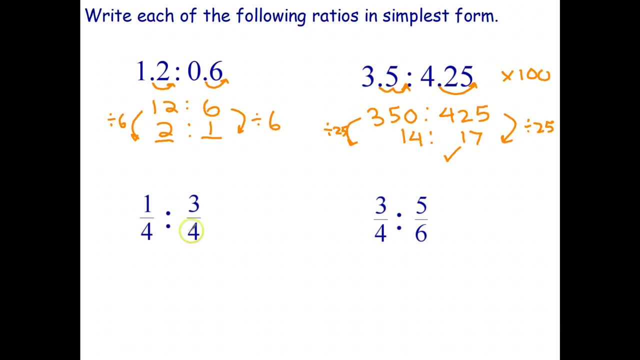 Okay now if you have fractions, if they already have a common denominator, you can just say: therefore, the ratio one quarter to three quarters is just one is to three. So effectively you can ignore the denominator, or another way of thinking about it. 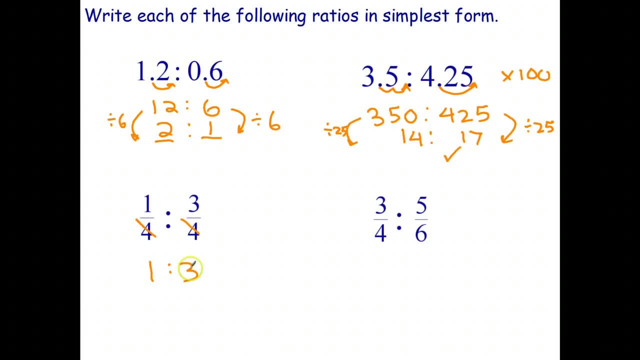 Multiply both of those fractions by four and you'll get that ratio. If the fractions don't have a common denominator, well you can probably guess what you have to do. You've got to turn them into fractions with a common denominator. So in this case I can turn three quarters into twelfths by multiplying by three. 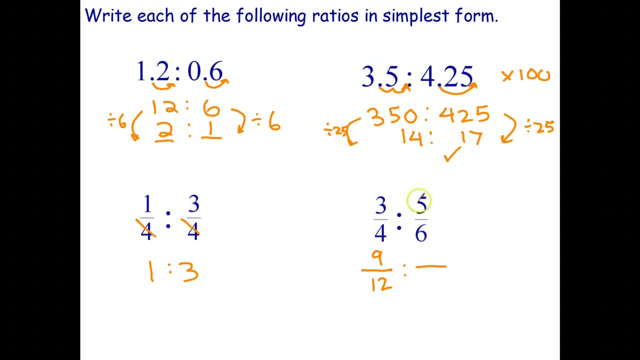 So that's the same as nine is to 12.. Multiply top and bottom by two, That gives me 10 is to 12.. My denominators are the same And therefore the ratio in simplified form is nine is to 10.. 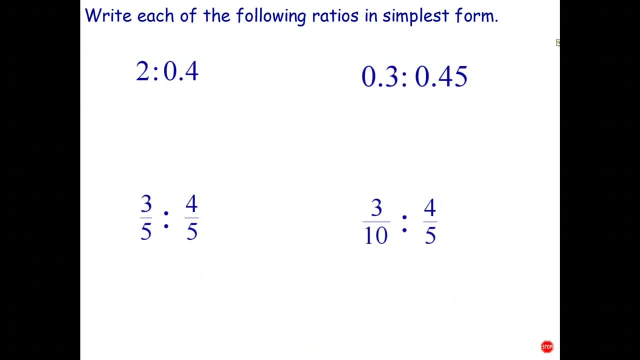 Okay, so I'm on the next page for you to try. Go ahead and simplify each of these ratios, please. Okay, welcome back. Let's see how you went. Okay, the first one. I've got one digit after the decimal point here. 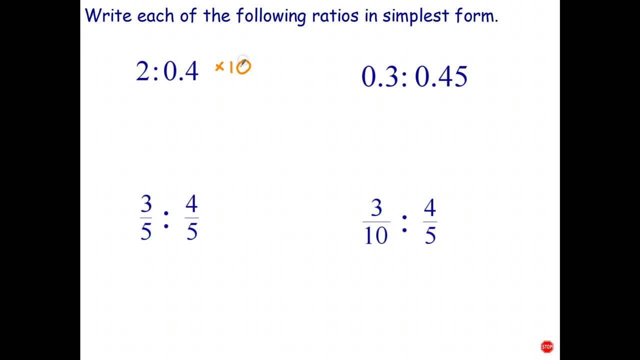 So to get rid of that, I multiply both numbers by 10.. Two times 10 is 20.. Point four times 10 is four. So the ratio is 20 is to four. Four is the highest common factor. So I'm going to divide both numbers by four. 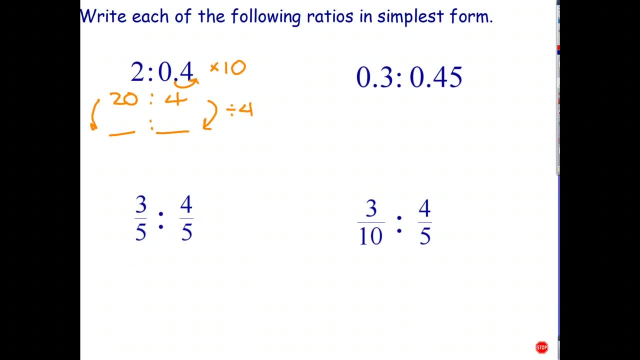 Oops, that was a bit of a dumb thing to do. Let me just go get that line back, if I can. There we go. So I shouldn't have probably written over there. I'll just leave that 20 divided by four is five. 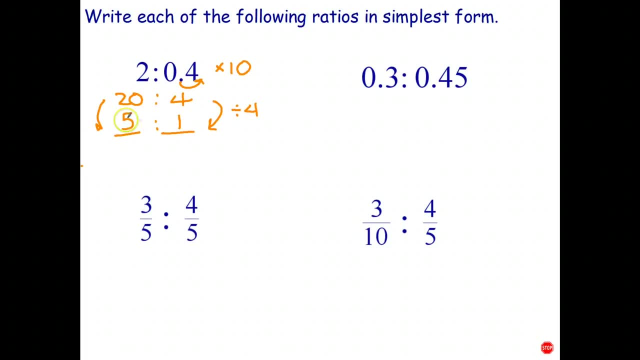 Four divided by four is one, And the simplified ratio is five is to one. Here I have to multiply by 100, because I have two decimal places, two numbers after the decimal point. So I divide: Here's 100 times 100.. 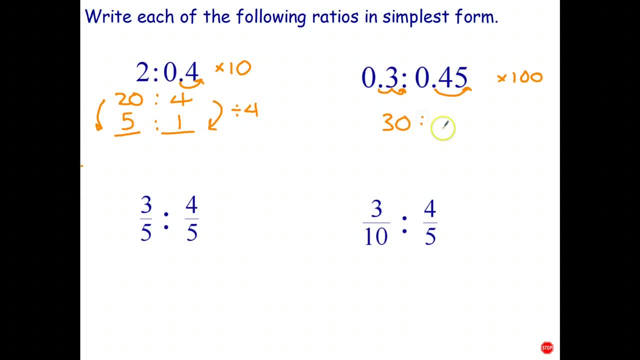 And that's going to give me: 30 is two 45. Now I know that 15 goes into each of those, So I'm going to divide by 15.. I'll just write it on one side. Nothing wrong with that. 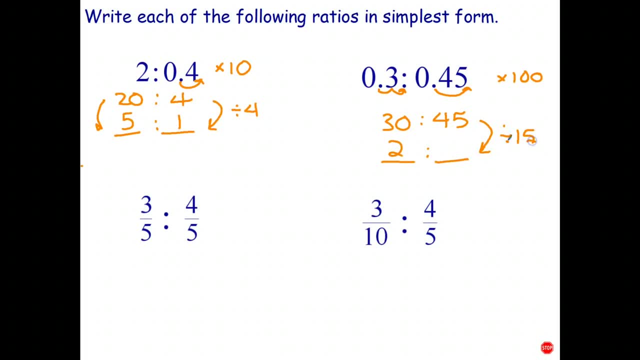 30 divided by 15 is two, 45 divided by 15 is three, And the simplest ratio, or the way to simplify that ratio being two, is to three. OK, This one's fairly straightforward, because my denominator is five. In simplest form, the ratio is three is to four. 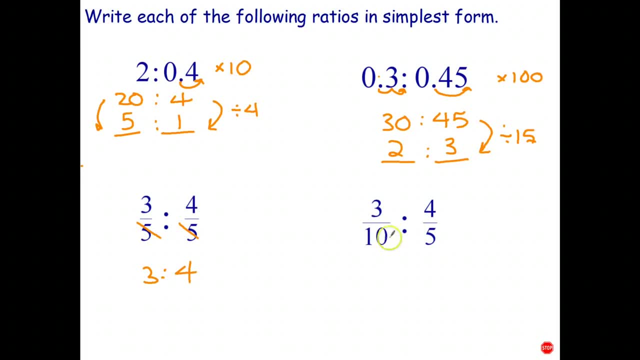 And for this one I've got to get a common denominator of 10.. Well, this one already has a denominator of 10. So that needs nothing done to it. Multiply top and bottom by two, That gives me eight is to 10..